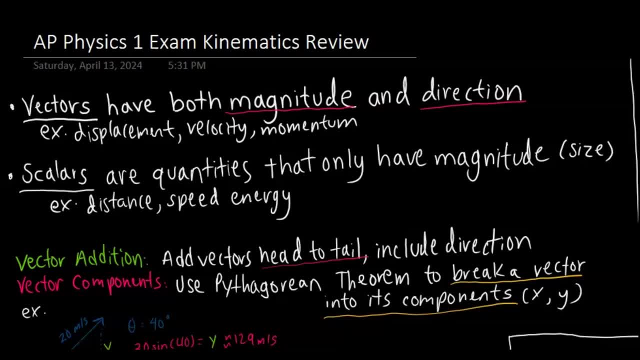 physics foundation, And so we need to be able to recognize the difference between a vector and a scalar. So vectors have both magnitude or size and direction. So example of that would be displacement velocity, momentum. Now scalars are quantities that only have magnitude, and so 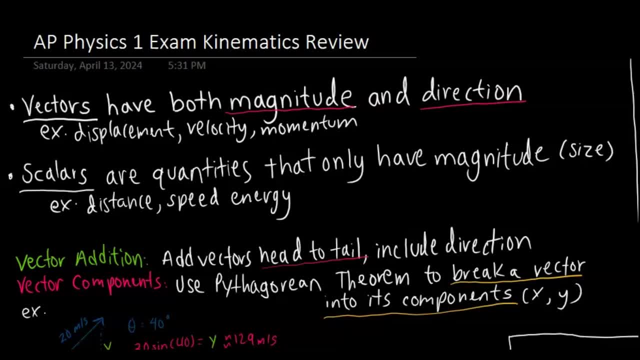 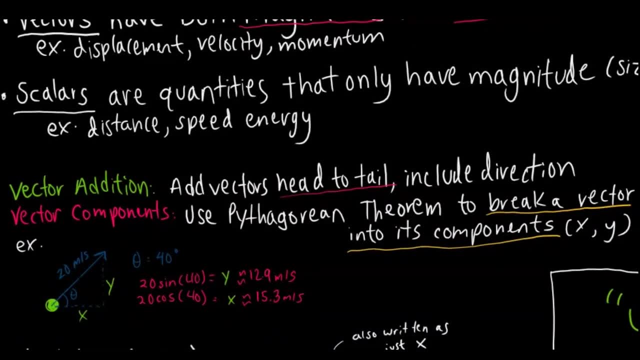 that's stuff you don't have to specify direction for, like speed, energy, distance. So now, when you're adding these vectors, there may be some problems that show up in terms of testing your knowledge on adding vectors. You need to add vectors from head to tail and also. 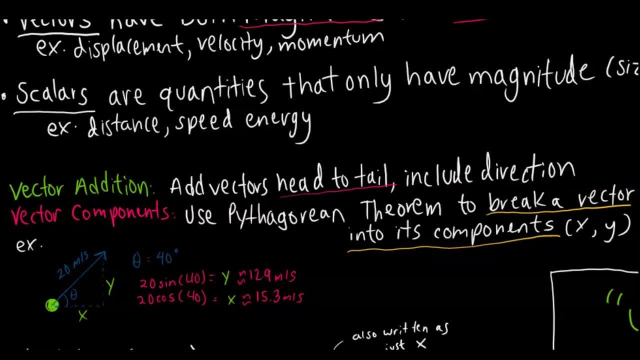 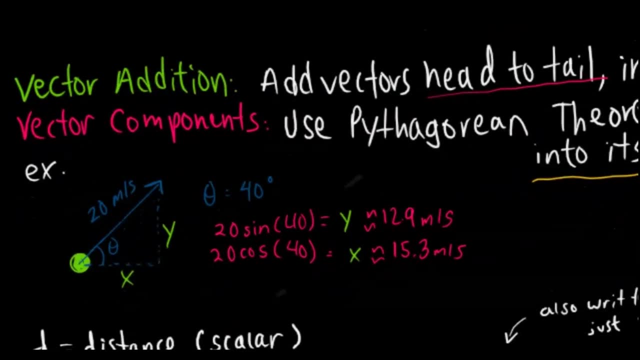 include the direction, And the more important part of vectors in terms of the actual exam is being able to break them apart into components. So once you break them apart into components, you want to use the Pythagorean theorem to analyze it. So here's an example. Let's see we had a ball. 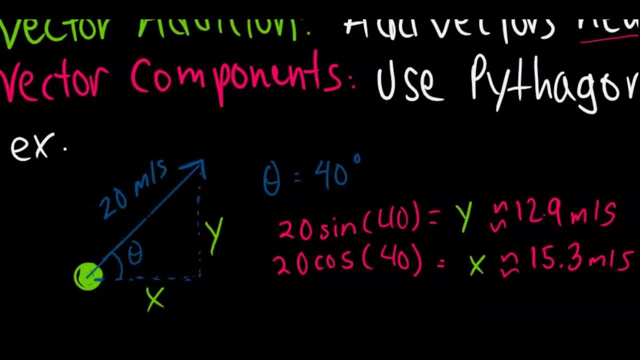 launched with 20 meters per second of initial velocity, Because the force of gravity is acting upon the y direction but not the x direction. it affects it differently. So in order to analyze its motion, what you need to do is break it apart and do its components. You know the angle measure. 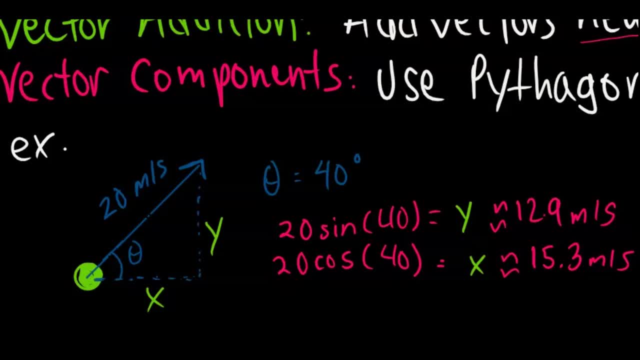 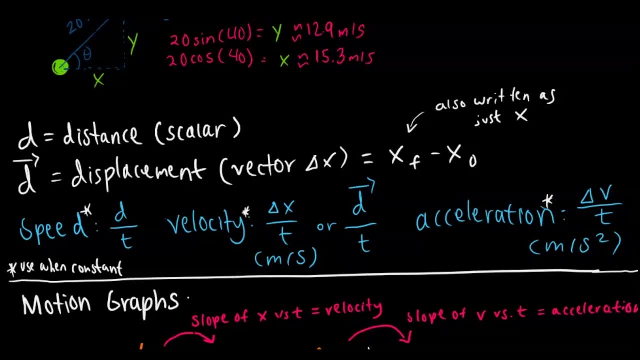 presumably, and then you can just use trach to find the different velocities, just like that. All right, so now let's get into some of the actual motion stuff for kinematics. So the first one is the distance, which is represented by d, but sometimes it can just be written as d, for 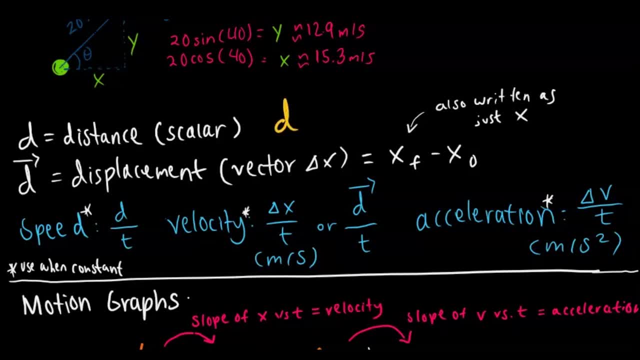 displacement like this. So sometimes you can write displacement like that with um like that Um. but more traditional way to represent displacement is just d, with an arrow over it to show direction. So distance of scalar. Well, displacement is a vector and that represents change in position, right? 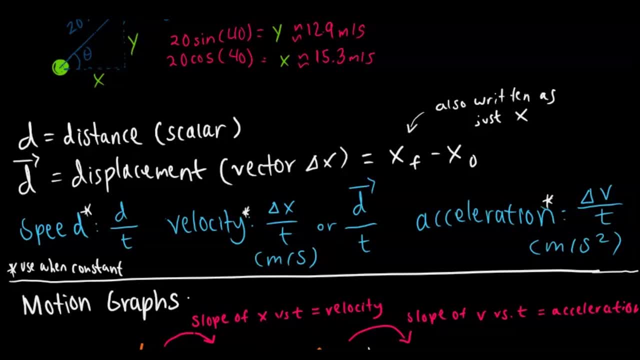 So that is otherwise known as final position versus minus initial position. so easy way to think about that is: let's say you had a guy and he walked for 10 steps and then walked backwards five steps. his total distance traveled would be 15 steps, but his displacement, which is change in position. 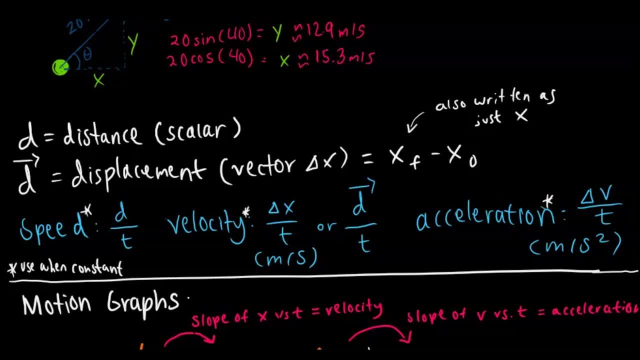 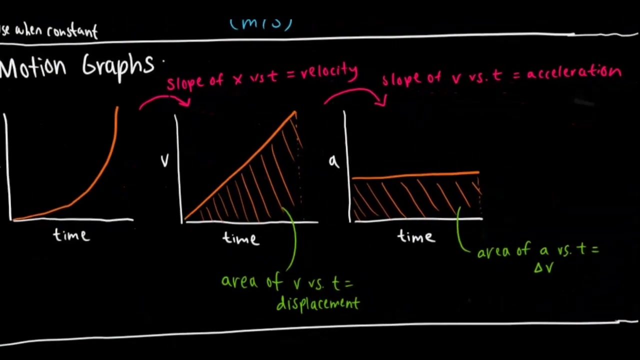 would be five steps. speed is distance over time. velocity is change in position over time or displacement over time. acceleration is just how fast your velocity is changing over time, and there are the different units, which are represented as meters per second for velocity and meters per second squared for acceleration- motion graphs. you need to know how to interpret. 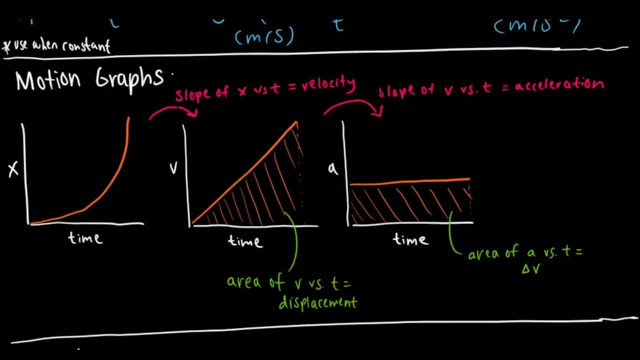 these graphs- and i just have one example here- where you can see the position is exponentially increasing, right? so, in contrast to that, you have that velocity over time graph that's going to be increasing at a constant rate, and so, because you're increasing your velocity each increment of time, what you're going to get is the exponentially increasing position. 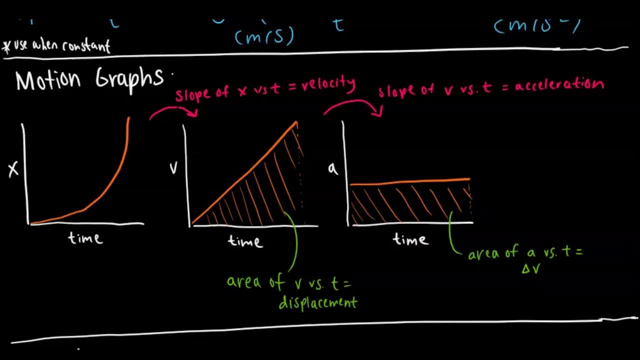 right. you're getting faster each time and therefore your position is going to change exponentially. now your acceleration is based off your velocity versus time graph, just like your velocity is based off the position over time graph, and that's represented by the slope. so the slope of the position versus 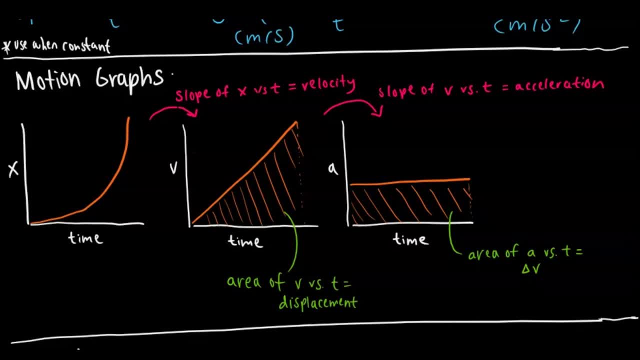 time graph is your velocity, the slope of the velocity versus time graph is your acceleration, and then you want to work backwards from that, which is analyzing the area under the curve. so the area under the curve for this acceleration would be change in velocity and the area of 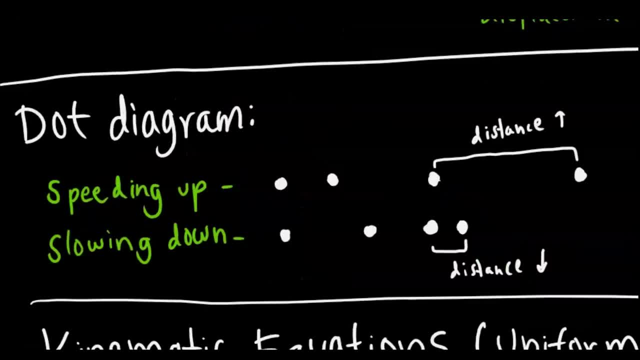 velocity over time, uh, would represent your displacement. all right. so here's another thing you might want to take note of, which is the dot diagram, so being able to differentiate between um the position of the object, whether it's speeding over time, or velocity over time, up or slowing down. so let's say you had like a motion camera that captured the position of the 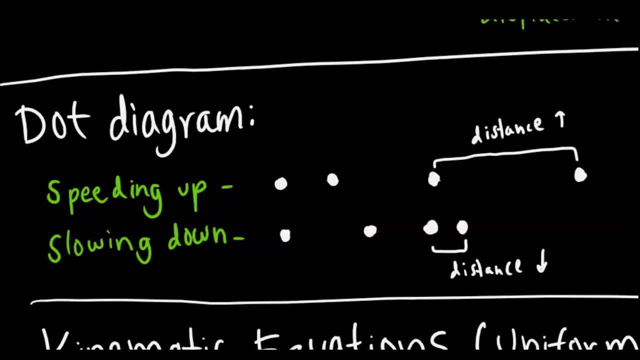 object every increment of seconds, like every one second, so you're able to tell whether it's speeding up or slowing down. so the first example: you can see how it's speeding up because, since it's going faster right in that same amount of time when it takes that picture on the distance. 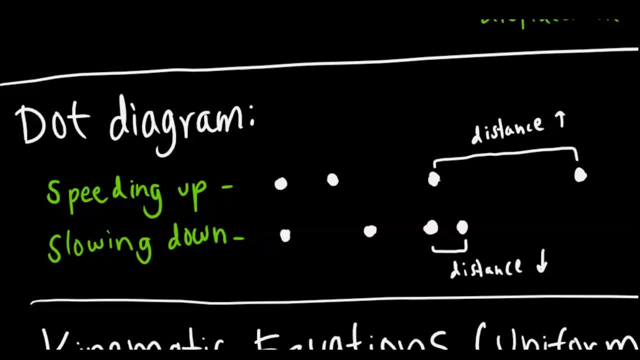 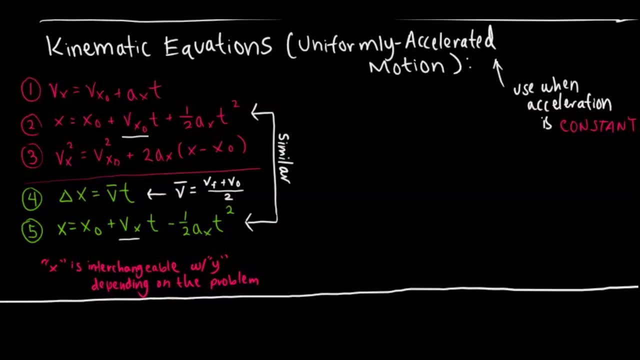 it travels is going to be greater and, in contrast, when it slows down, that distance is going to decrease. okay, so now we want to look at the kinematic equations, and these are the uniformly accelerated motion equations, and so you want to use these when the acceleration is constant, if 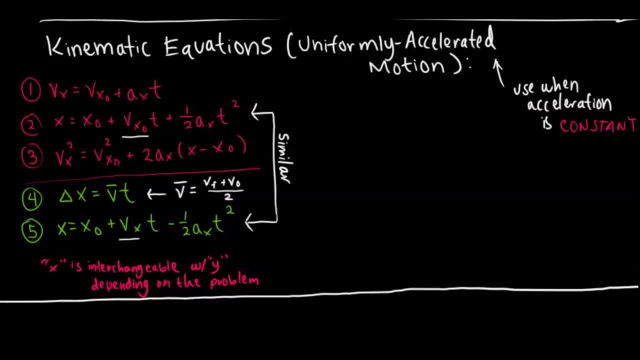 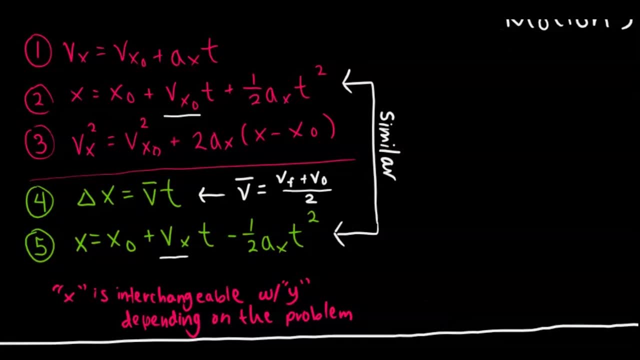 acceleration isn't constant. what you can do is just break the problem apart to analyze it in parts where the acceleration is constant. so the first three here are on your reference table, but the two in green are not, and those would probably be helpful to memorize. um. so what you'll find is that 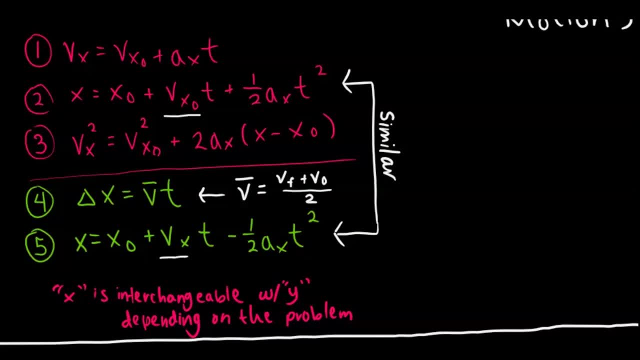 two and five are pretty similar in terms of uh the content. the only difference is that the uh initial velocity is swapped with the final velocity, um. and to make up for that, instead of plus one half a t squared, it is minus one half a t squared. and another thing thing to know about: 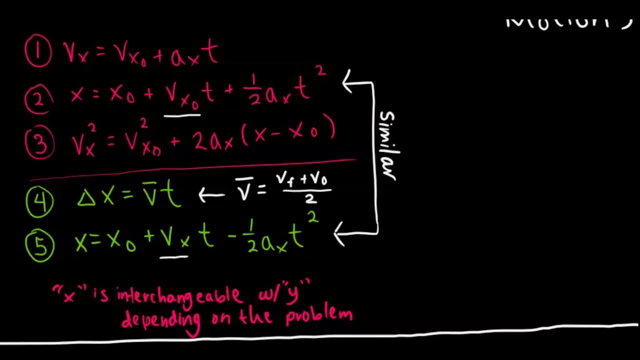 these equations is basically: if you have the unknown variable and you know the other three or two variables, then you can plug it in to solve for those and that is sort of the basis of kinematics. and x in these examples can be interchangeable with y. it just shows the 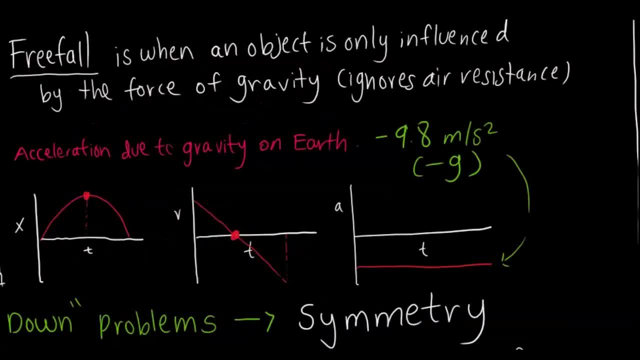 plane that is being analyzed and you'll see it in the practice problems. now we want to look at free fall, so this is when you just throw an object into the air and then you want to analyze its motion. or, let's say, you dropped a ball from a cliff, um, so this is where the only force acting 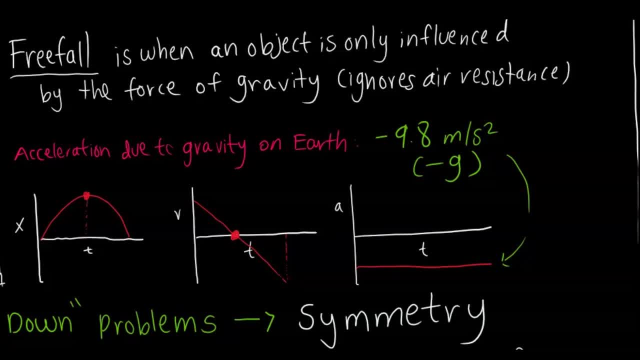 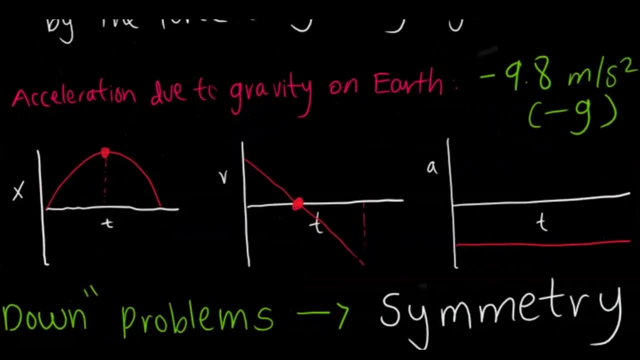 upon that object is the force of gravity and we're ignoring air resistance um and acceleration due to gravity on planet earth. it is negative 9.8 meters per second squared. it really is 9.8 meters per second squared, but because it's acting downwards it's negative little g. so these are the motion graphs for it. you can. 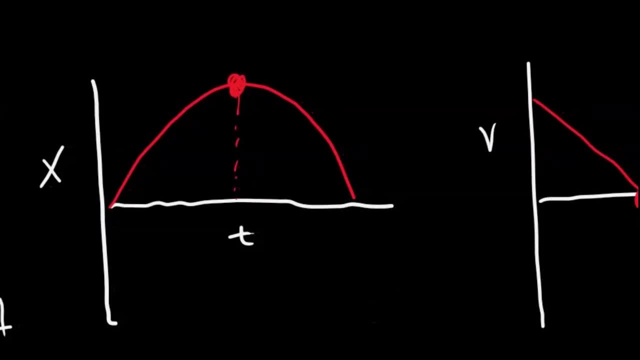 see how- um, let's look at this first one, where there is position over time. this is something that would be represented by, let's say, you throwing a ball straight up and then it comes down. so you throw it straight up and then it reaches its apex and then comes down to its. 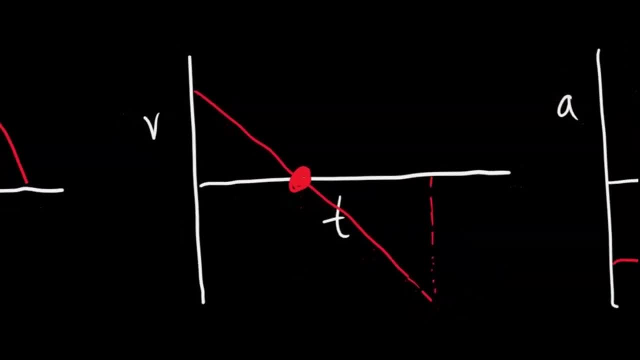 initial position and the velocity over time graph you can see is where you give that ball initial velocity. but then what happens is that, since the only force acting upon it is negative g right acceleration is going to be: um, sorry, that velocity is going to be positive, but it's going to. 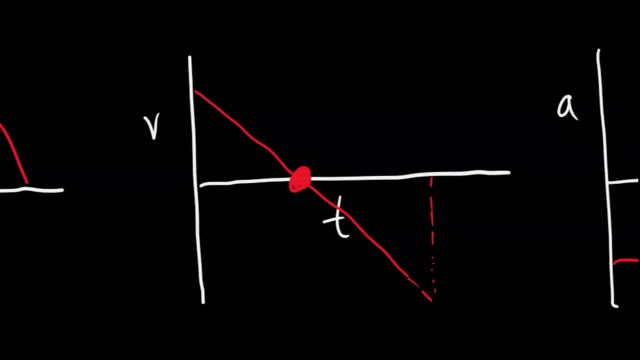 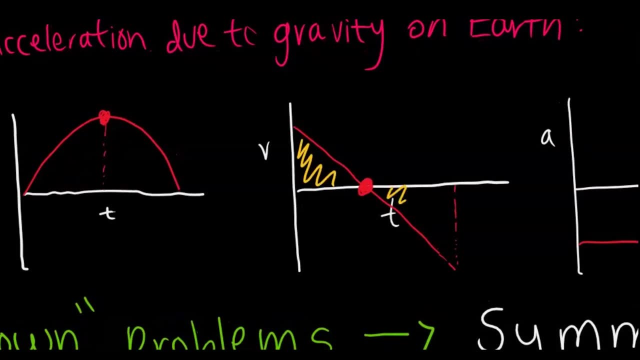 be decreasing right until it reaches zero, which is when it hits its apex, and then it's going to go negative and start falling back down. you can see how the areas are equal to each other. so this area right here is equivalent to this area right here, which shows the total change in displacement. 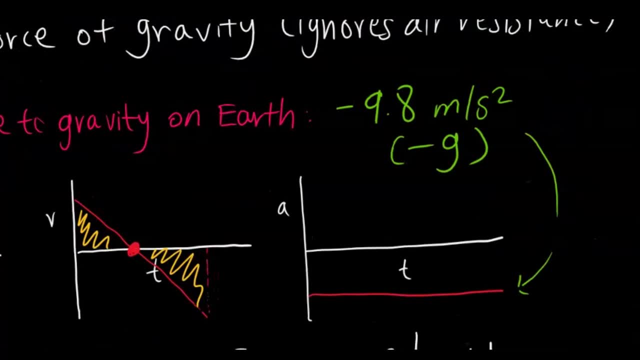 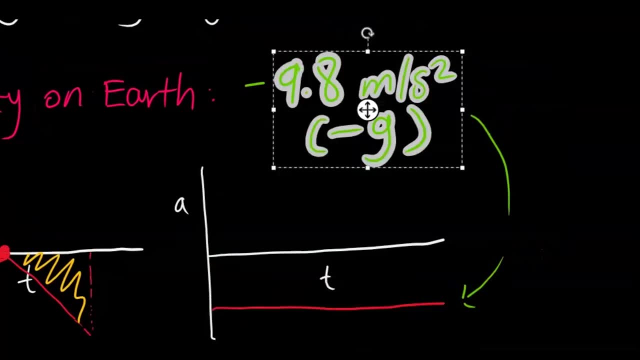 which would be zero if the ball came back down to you, and then the acceleration due to gravity is the only force acting upon it and that's why it's just a straight line in the negatives which shows it's being affected by that um negative 9.8 meters per. 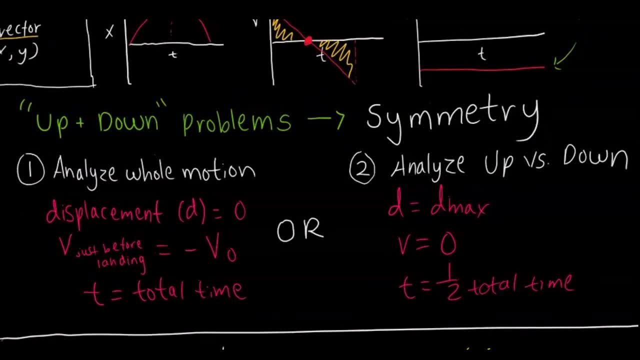 second squared. all right. so the other thing regarding free fall is up and down problems, and so we already talked about that symmetry that you're going to see. um, but there are two strategies you want to use when analyzing these problems. you can either analyze the whole motion. 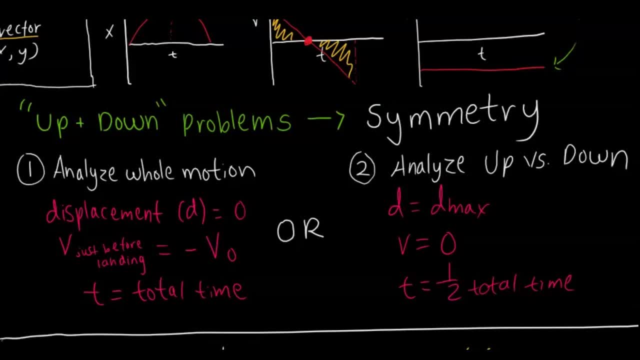 in which the displacement would be the same, or you can either analyze the whole motion, in which the displacement would be zero because it came back down. the velocity just before landing is the negative of that initial velocity and then the time is just the total time it took for the 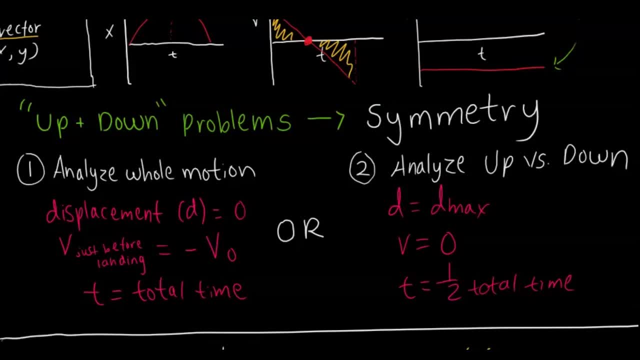 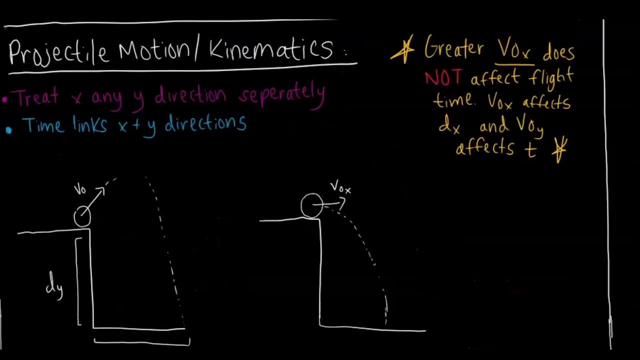 entire motion, or you can just analyze just the up portion or just the down portion, in which the displacement would be max. the velocity would be zero, since when it reaches its apex that would just stop, and then time is just half the time. all right, so the final thing we're going to cover is 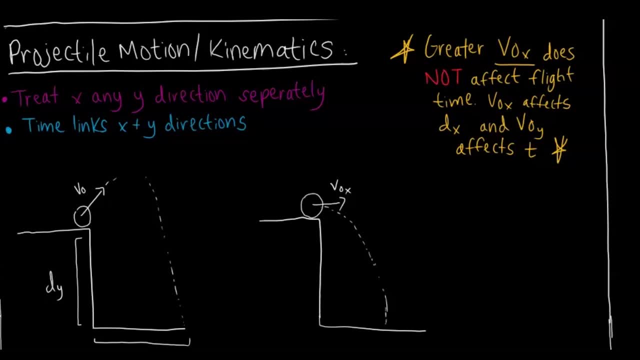 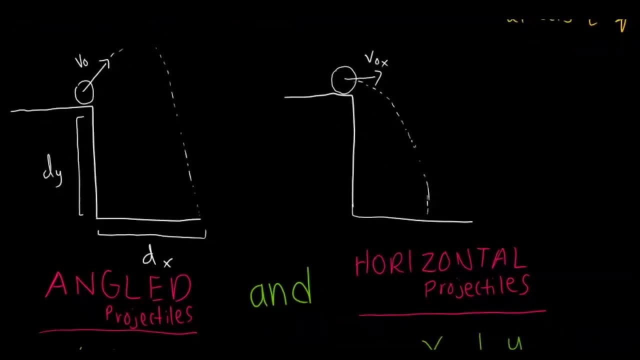 projectile motion in terms of kinematics. So there are two types of projectiles. You're going to have angled projectiles and horizontal projectiles. So when it's angled, it's launched at an angle into the air, And when it's horizontal, it's just launched at 90 degrees flat. 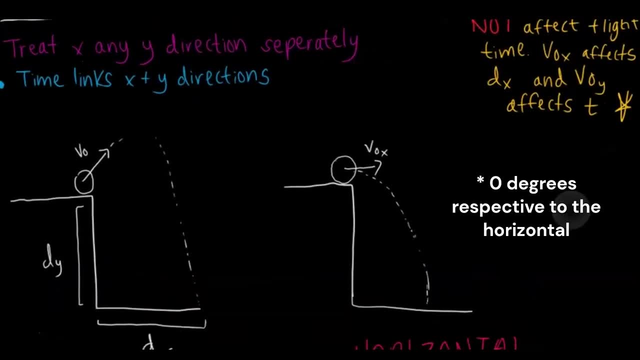 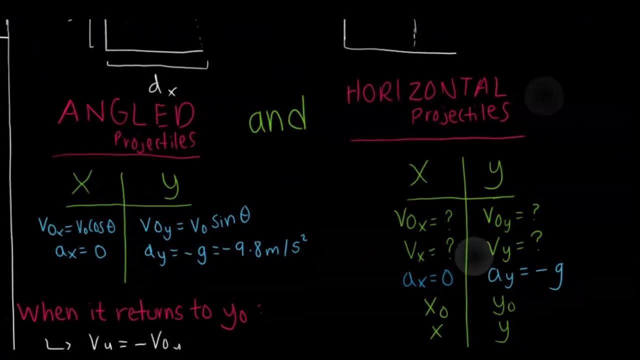 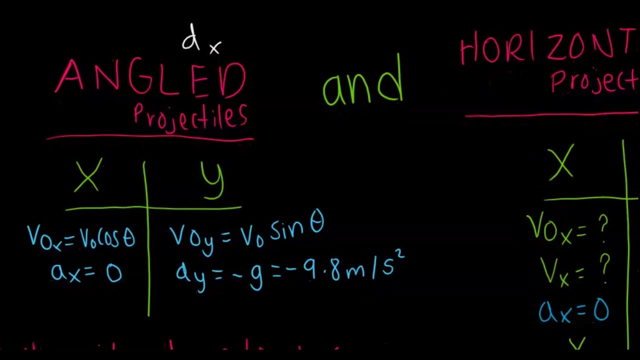 given an initial velocity as well, And that initial velocity is going to act in the X direction. So these are a couple universal laws that would apply to these projectiles. So for the angled projectiles, what you're going to do is break that velocity into its component right. 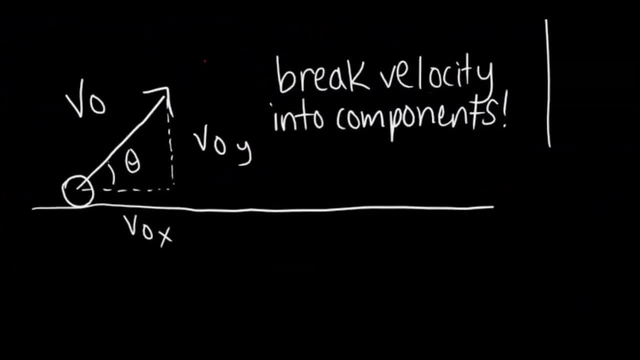 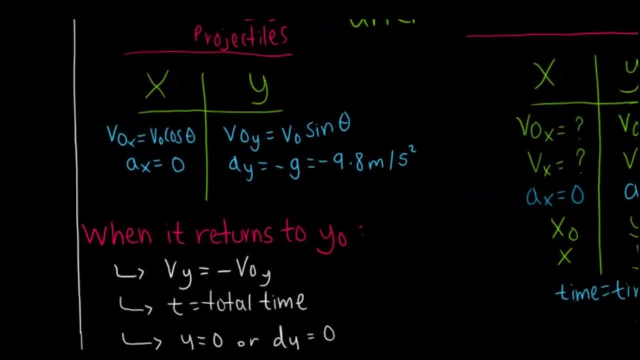 Just like what we said before, we want to break that initial velocity right here into its different components using trig. So once we get those values, there are a couple ways to analyze it And I'll get into that in a little bit. But now I want to look at the horizontal projectiles. 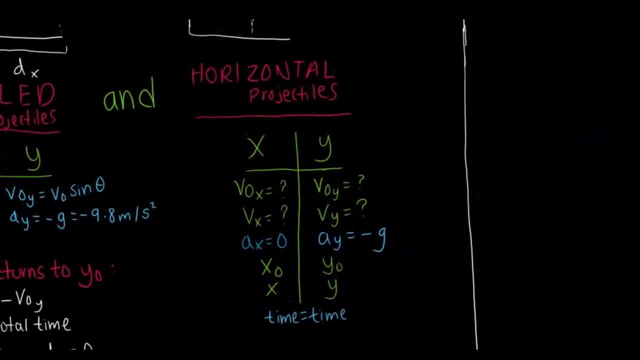 So your initial acceleration in the X direction would always just be zero, right, Because after you give it the initial velocity, there's nothing active And the X direction, since some of all the forces in the X direction would be zero when it's in the air.